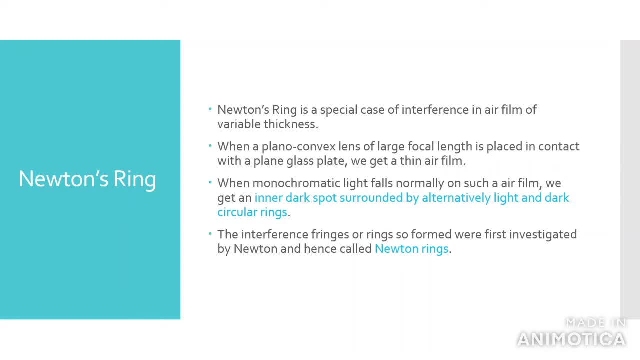 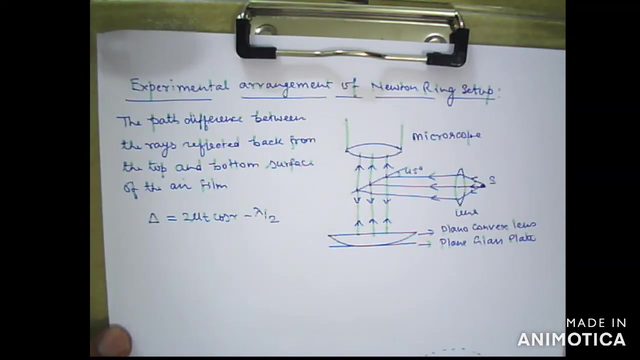 So this is the basic theory of the Newton's ring. Now we will discuss the experimental setup and the condition for the path difference, and then we will get the condition for the diameter of the dark and bright ring. We have prepared the experimental setup of Newton's ring. 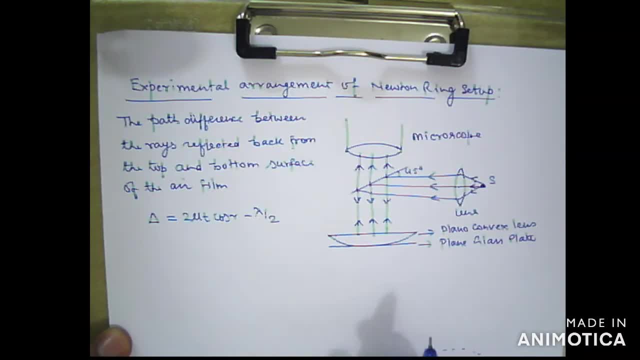 So first of all, let us understand the experimental setup Here. you have placed a plain glass plate at the bottom. On this plate you have placed a plano-convex lens whose radius of curvature is large, near around 1 meter. So if we talk about the diameter, then the diameter of this plano-convex lens is around 2 meter. 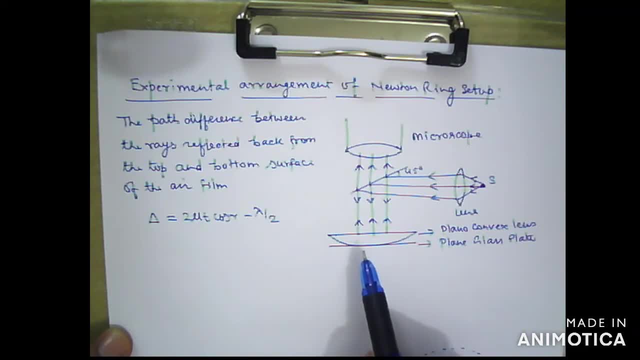 So it has a very large radius of curvature. So when you put this plano-convex lens over this plain glass plate, you will get the air film between the plain glass plate and this plano-convex lens. Now, here we have placed a monochromatic source from where the light is coming. 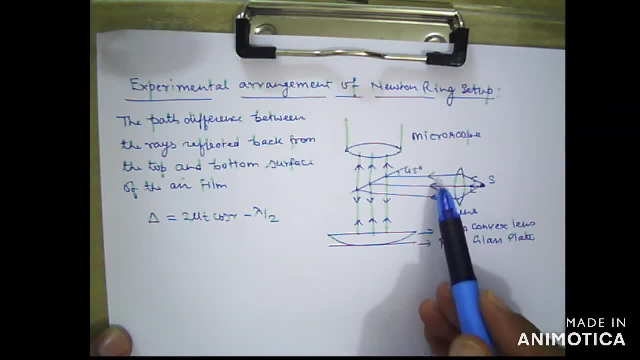 After passing through this convex lens, then the radius will be parallel to each other. When this radius falls on this glass plate at 45 degree, then from here it will reflect at 90 degree. Incident light goes through. If this angle is seen, then this angle becomes 90 degree. 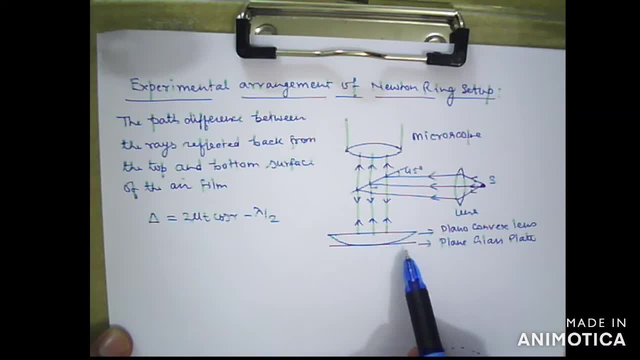 So these rays will incident on this plano-convex lens and plain glass plate And they will reflect from the bottom of the air film and the top of the air film. So when they will reflect from this air film they will superimpose on each other and will produce the Newton's ring fringes. 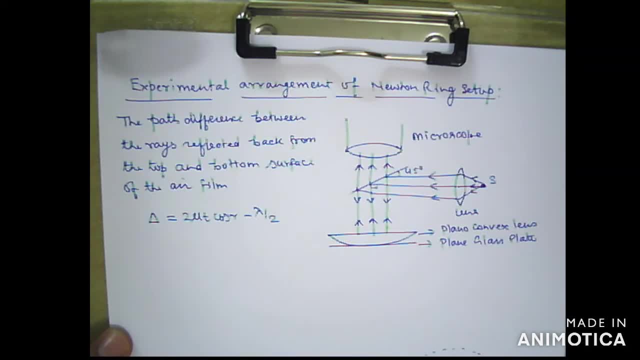 Now, here we can understand why Newton's ring will be formed, The reason why the dark center will be formed above this contact point. I will tell you further in this. And what we are seeing here is that the thickness of this air film is increasing gradually. 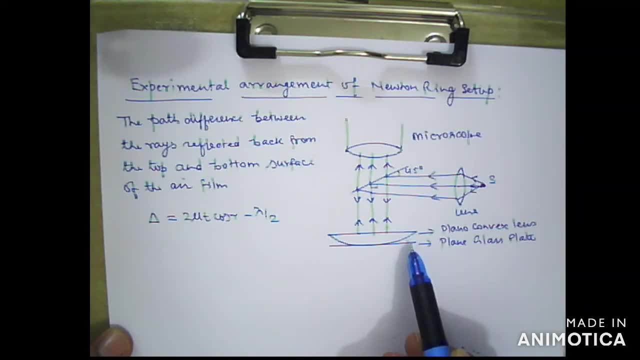 So if we talk about the constant thickness, then at any point if you calculate the constant thickness, as you have seen here, then this thickness will be constant in the whole circle. This means that if the path difference is calculated, then if you calculate the path difference, 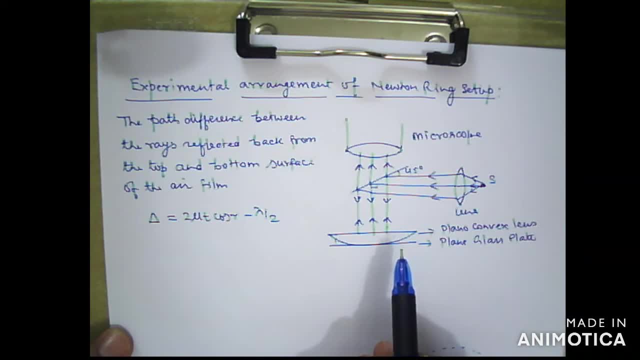 then the path difference for the whole circle will be constant. So at the same time it will satisfy the condition of dark and bright, So you will get the alternatively dark and bright fringes. So this was our experimental setup, which you might have understood. 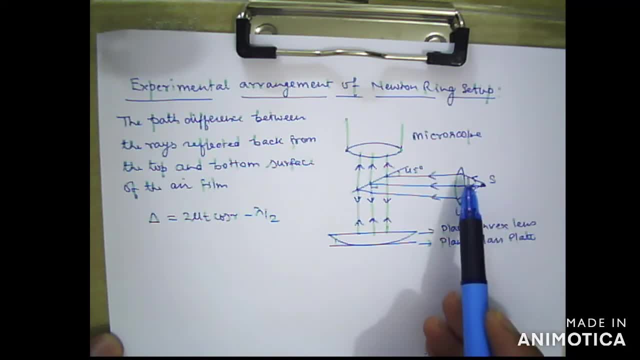 It is simple: nothing much. A plain source is kept, a convex lens is kept in front of it. After the rays come out from here, an incident occurs on a plain glass plate. After it reflects from here, this plane of convex lens and a plane of glass plate, incident occurs. 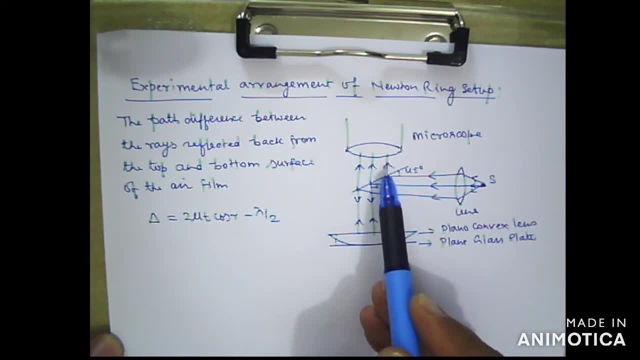 both are reflected from here And when it is going back and forth. here they become superimposed and form interference fringes, And these fringes can be observed by the help of the microscope. In the last lecture we had seen that we had calculated the path difference for thin film. 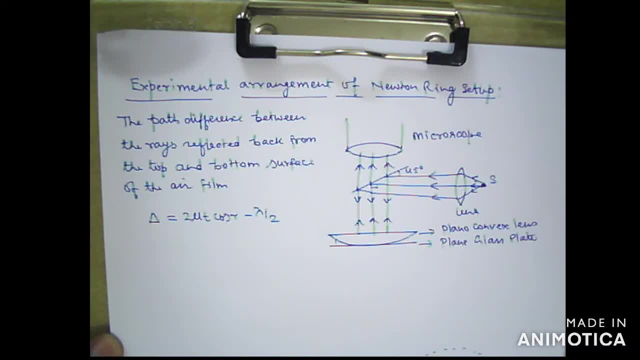 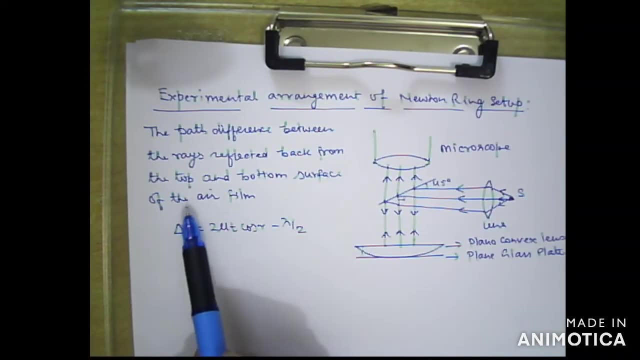 So I had also told you that we are going to use the same path difference here also. So the path difference between the rays reflected back from the top and bottom surface of the air film is that delta equals to 2 mu t, cos r minus lambda pi. 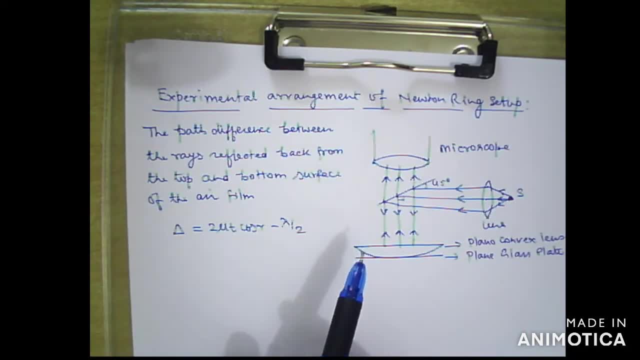 So here we have considered the same path difference of thin film, and now we will use this path difference to calculate the condition of dark and bright. Now let us talk about what is the view. Mu was the refractive index of the uniform thickness glass plate. 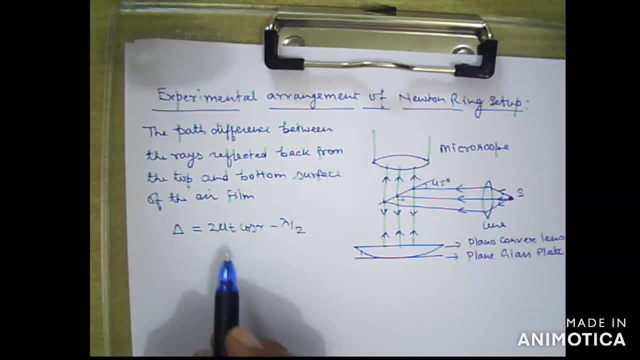 But in this case our medium is not glass, our medium is basically the air. So what can we say here? 4 air medium mu equals to 1. For air, the value of refractive index mu will be 1.. And if we say that? 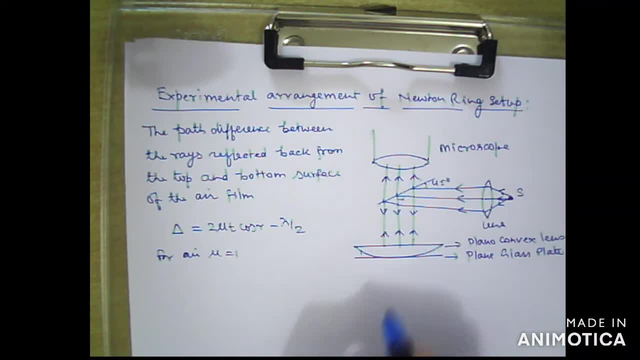 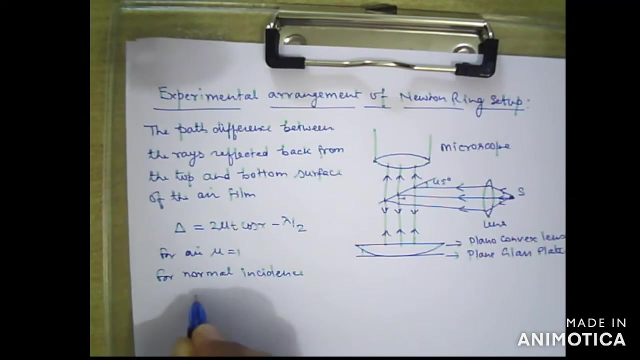 if our lights are normally incident on this plane of convex system, then in the case of normal incidence the angle of incidence will be I0, then the angle of refraction r will also be 0. So here you can write: for normal incidence, r equals to 0,. so cos r equals to 1.. So if you use these two conditions in this equation, number 1,, then what will be our path difference? So path difference delta equals to 2t minus lambda by 2.. This will be the path difference for the Newton's ring fringes. 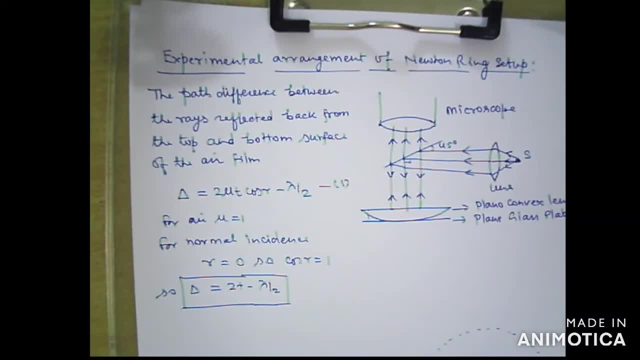 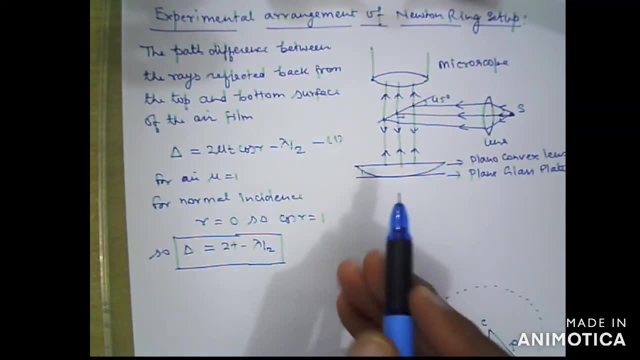 Now, if you have this path difference which will satisfy the condition of dark and bright, then it will be in the whole circle, as I told you earlier, because the thickness of the air film, if I talk in a whole circle like here, is t and here is the same thickness. 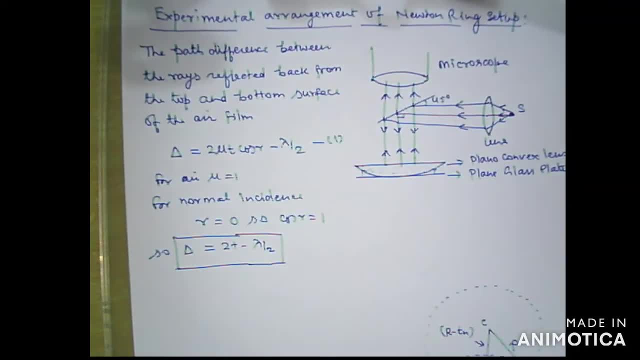 then this will be a whole circle. So for this whole circle the thickness will be constant. So here, in this expression where you have drawn the path difference, in this path difference the variable quantity is equal to t, Lambda is fixed. 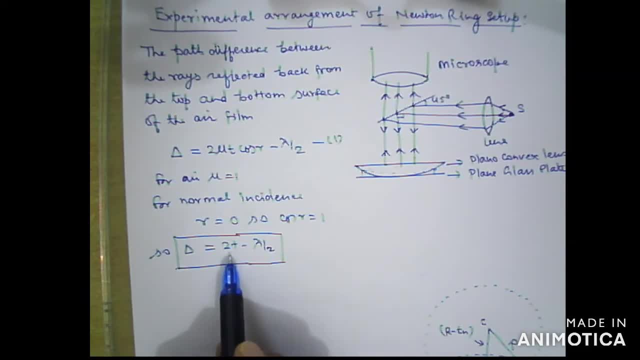 This means that the path difference depends on t, And if t becomes constant for the whole circle, this means that the condition for the whole circle is going to be satisfied together. So if we talk about the conditions here, then if you have read in the previous classes, 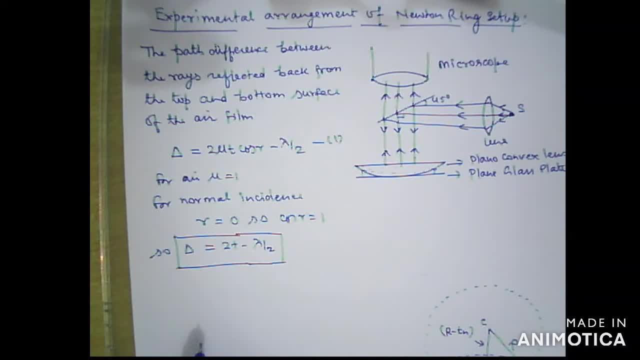 that if your path difference, which is delta, is equal to L lambda, then your bright fringes are formed Right. So let us first write the condition here. So when path difference delta equals to L lambda, we will get bright ring. 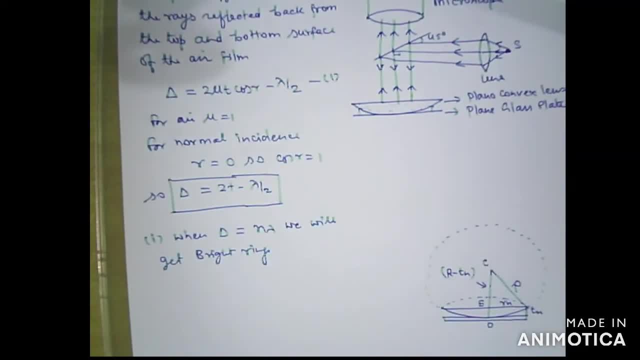 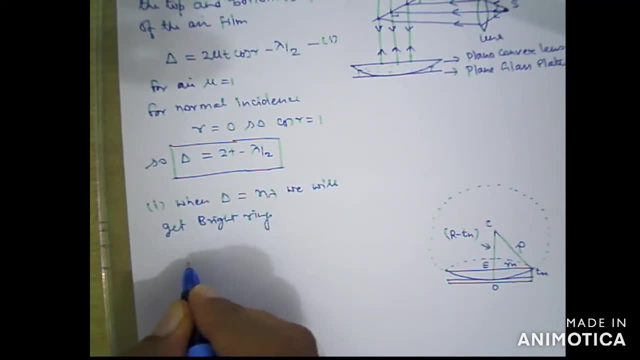 If our path difference delta is equal to L lambda, then what will we get? We will get bright ring. So let us keep the value of L lambda here. if the path difference, how much will it be? You will get 2t minus lambda by 2. 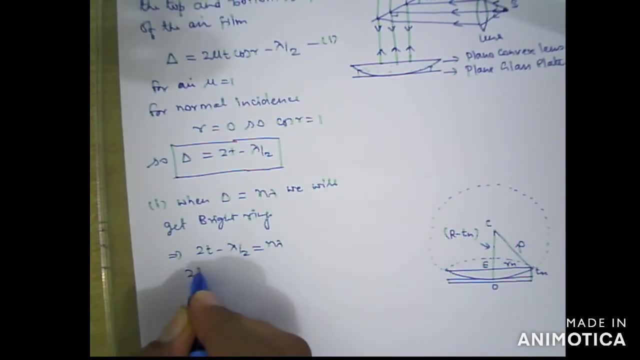 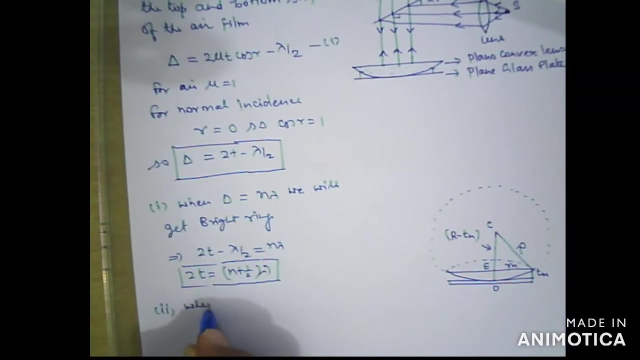 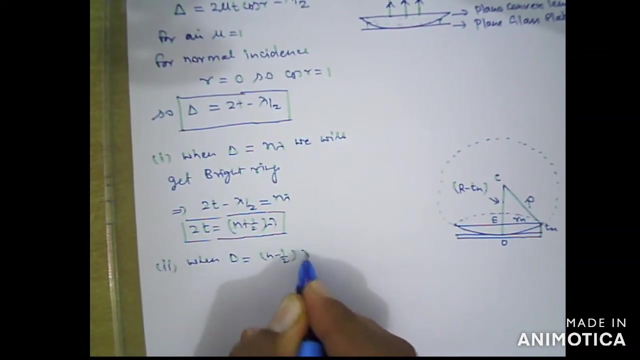 equals to L lambda, So 2t equals to L lambda. Here also the value of t is unknown. And if we go to the second case, when delta equals to n minus half lambda, we will get dark ring. If the value of delta equals to n minus half lambda, 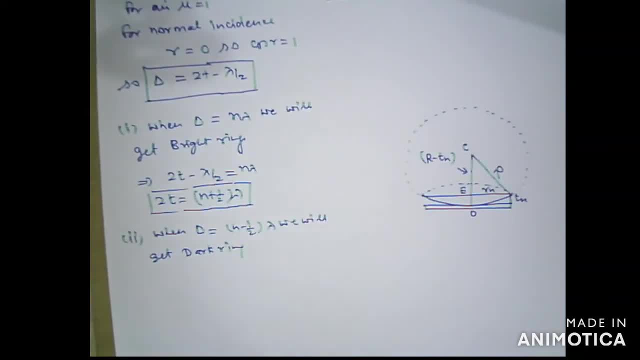 then in this case we will get dark ring. So let me put the condition here once. I will give the equation number 2 of this condition. So if I put delta here, we will get 2t minus lambda by 2 equals to n minus half lambda. 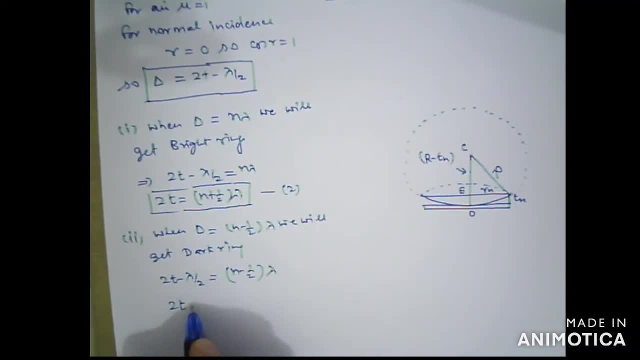 Half lambda will cross with half lambda, So the condition will be: 2t equals to L lambda, And this is the equation number 3.. This is the equation number 3.. But here we want to determine the value of the thickness of the air film. 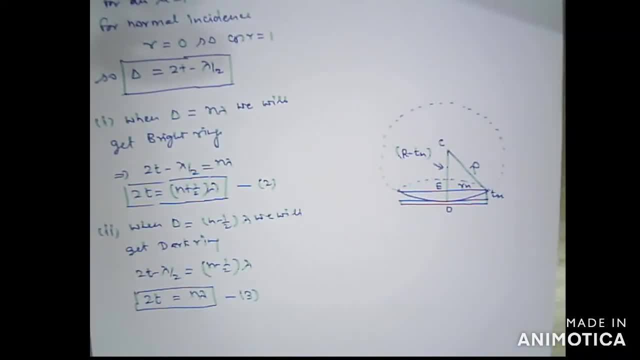 So to determine the thickness of the air film, we have made a diagram here. This is our plano-convex lens. There is a plain glass plate below The radius of curvature of this plano-convex lens. suppose I have taken R. 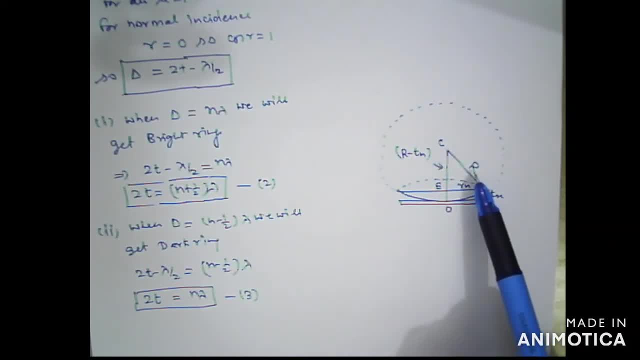 then the distance from C to here will be the radius of curvature R, And if I talk about O from C, then that will also be the radius of curvature R, But here the thickness at the extreme end. suppose I have taken Tn. 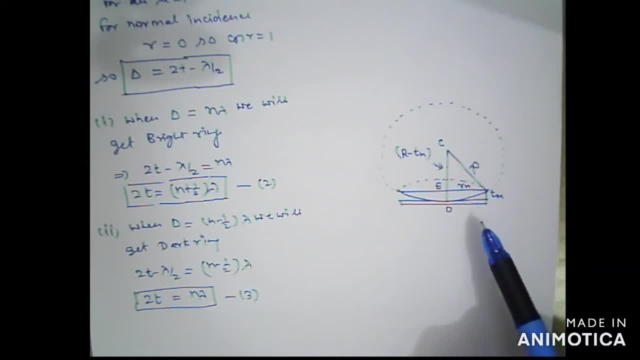 N is used in the subscript because we want to say that the ring of nth order is going to be formed here. So if this is Tn, then the distance from here to E will also be Tn, So the remaining distance from C to E. 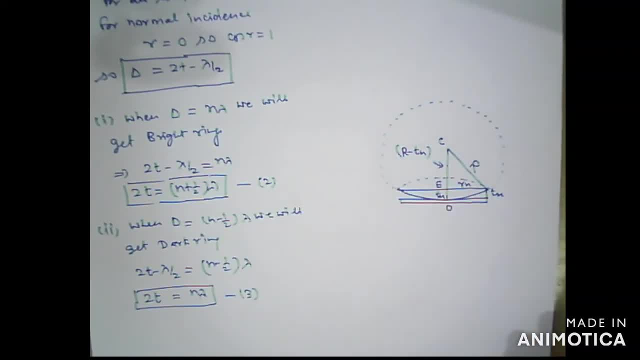 that will be the R minus Tn. Okay, And if here, at this position, the ring of nth order is formed and the centre of that ring will be E, then the distance from E to here will be the radius of the ring. 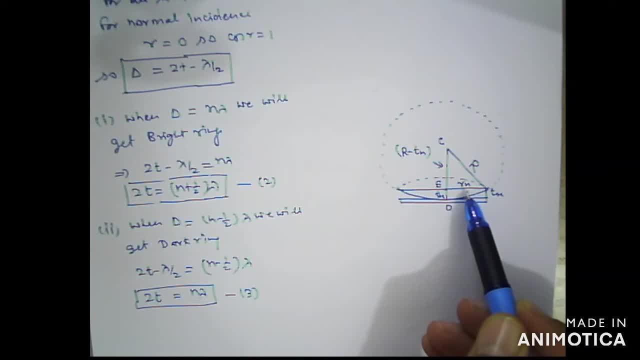 So if the order of the ring is N, then suppose the radius of the ring is Rn. So you must have understood this geometry. If we consider the triangle according to this geometry, suppose I assume this point as Q, so you can write here: 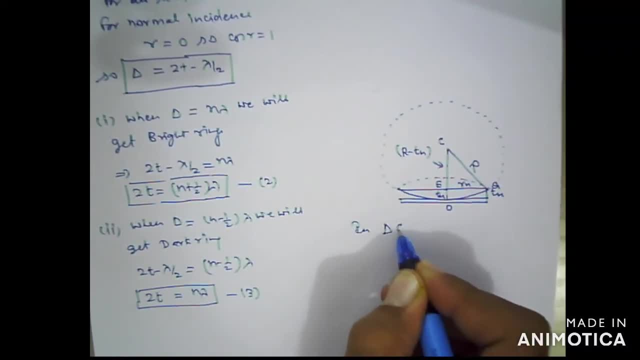 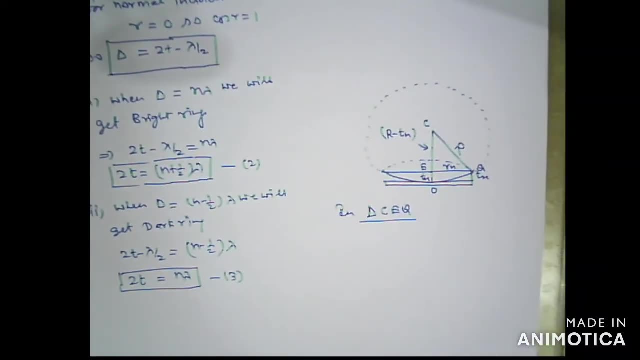 in triangle CEQ. If you consider the CEQ triangle here, then in the CEQ triangle we apply the Pythagorean theorem. So what will happen if we apply the Pythagorean theorem? CQ square equals to CE square plus. 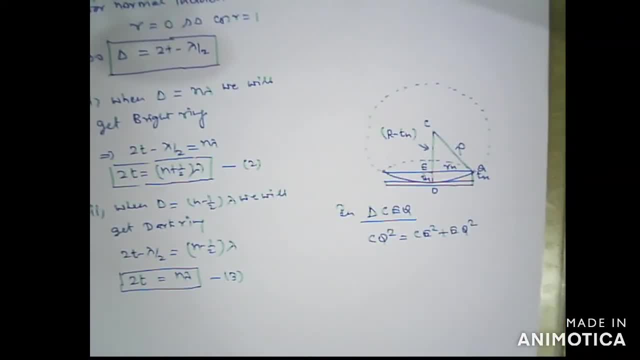 EQ square. This is done. Now what will be the value of CQ square from here R square And what will be the value of CE R minus Tn power square, And what will be the value of EQ Rn square? 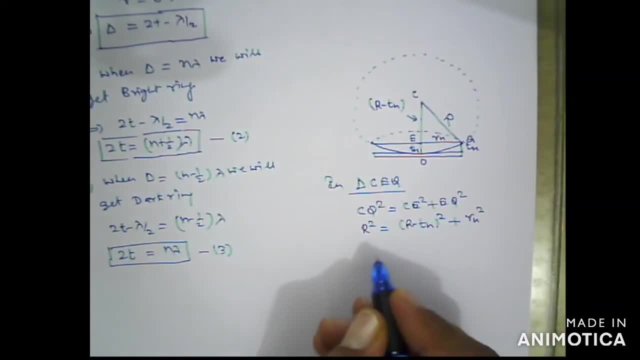 It is very simple. Now we will open its square once, So you will have R square equals to R square plus Tn square minus 2R Tn plus Rn square. Now, here R square equals to R square is cancelled. Now we can take an approximation here. 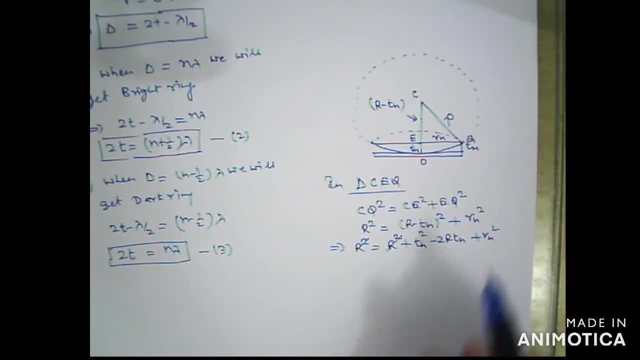 The approximation is, if you talk about Tn here, which is the thickness of this film, which is the maximum thickness here, the order of this thickness is of the order of 1 mm. So 1 mm is a very small quantity compared to this radius of curvature. 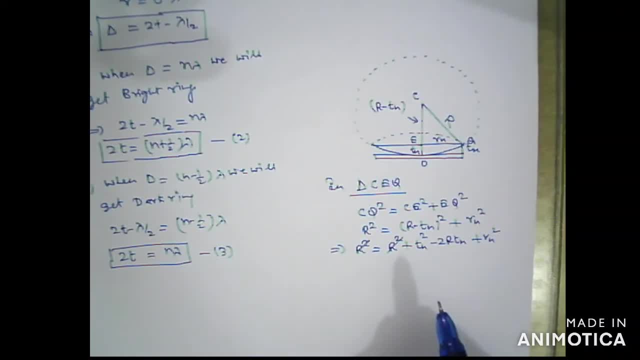 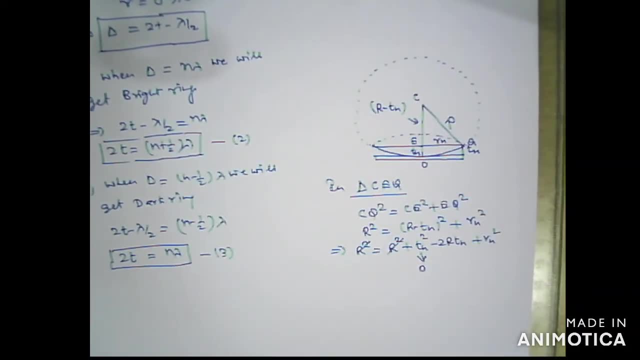 So if we square 1 mm, then again the quantity will go to the points, So you can take Tn square as a 0.. If we take Tn square as 0 from here, then what expression will we get If we solve this? 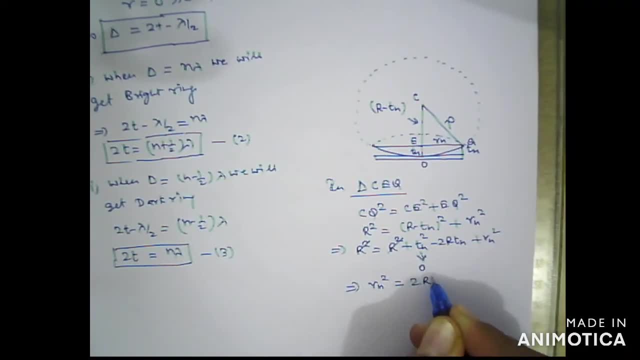 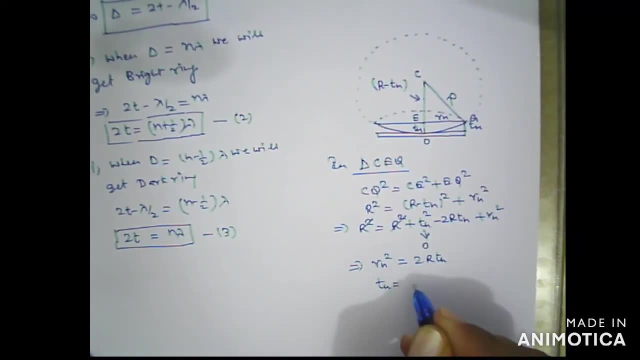 then you will get Rn square equals to 2R Tn. So from here, the value of the thickness Tn will be Rn square upon 2R. This is the value of the Tn. We have got the value of the thickness of this film. 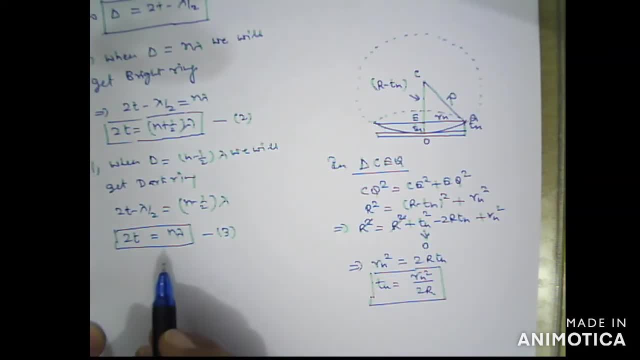 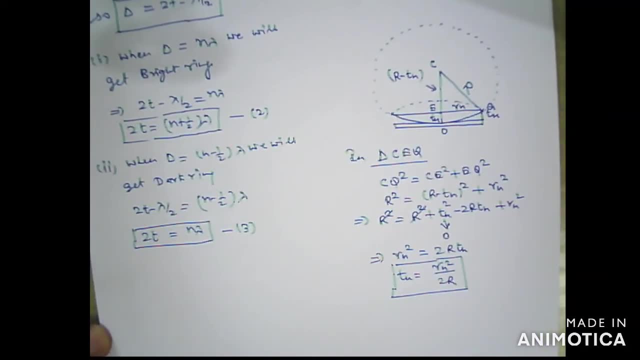 If I put the value of this thickness in my condition, then I will get the value of the radius of the nth order, dark ring or bright ring. Suppose I use this value in equation 3, then I will get 2, and how much will I put instead of T here? 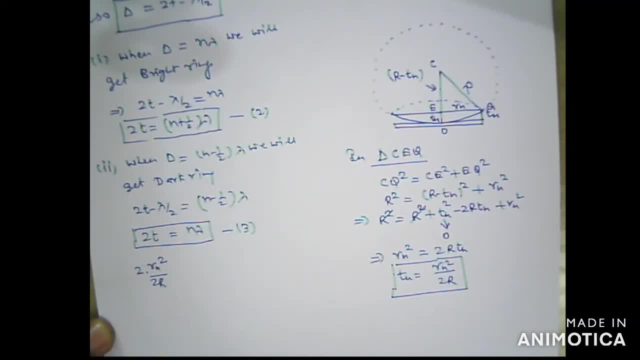 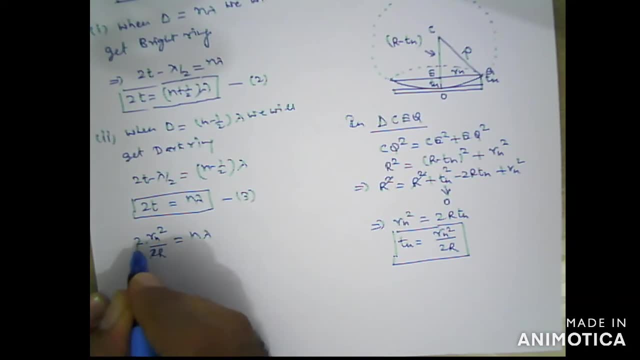 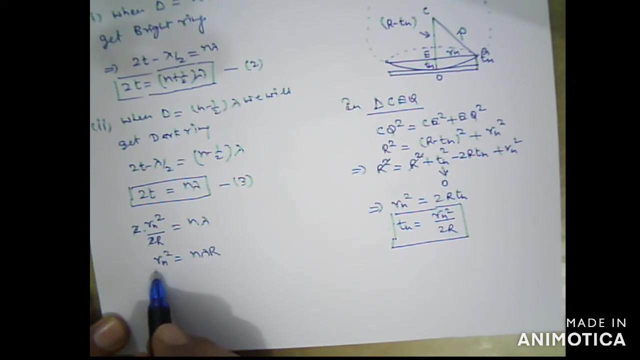 Rn square by 2R equals to n lambda. So if you cancel out 2 from here, then what is Rn square equals to n lambda R. If we want to write the diameter here, what is this? This is the radius of the nth order dark ring. 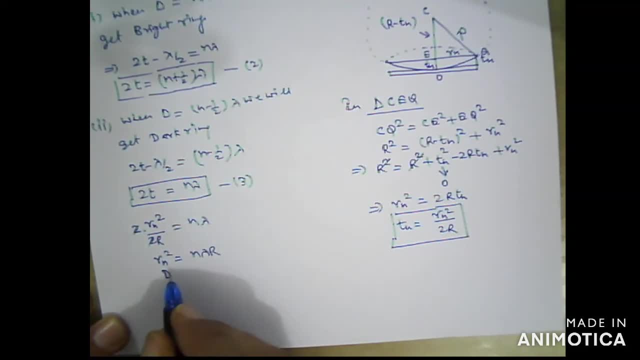 So if I want to write its diameter, then how much will be my diameter? If the diameter is written, then dn square equals to 4n lambda R, You will get the value of dn square. And if we want to get the value of dn, 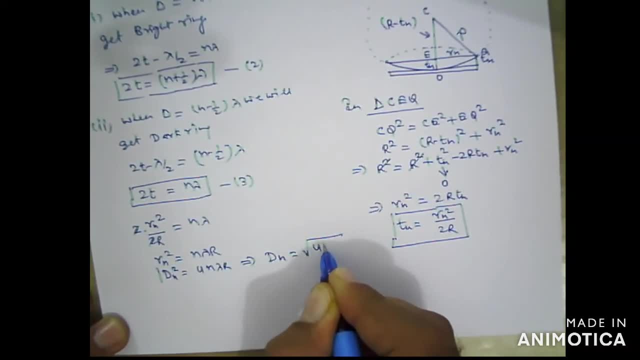 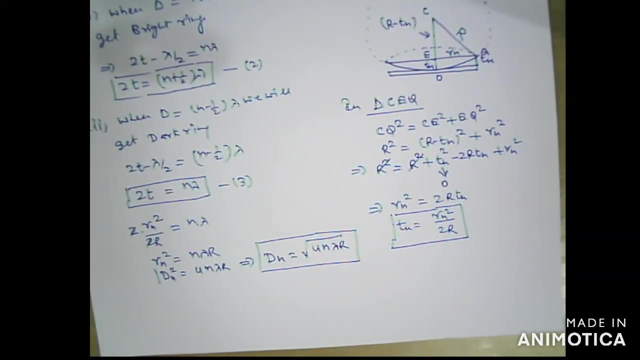 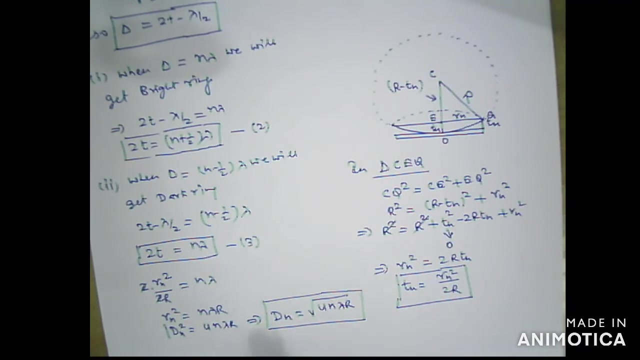 then how much will it be? Unroot 4n lambda R. This is the diameter of the dark ring. Similarly, you can determine the value of the diameter of the bright ring by putting the value of this Tn in equation number 2.. 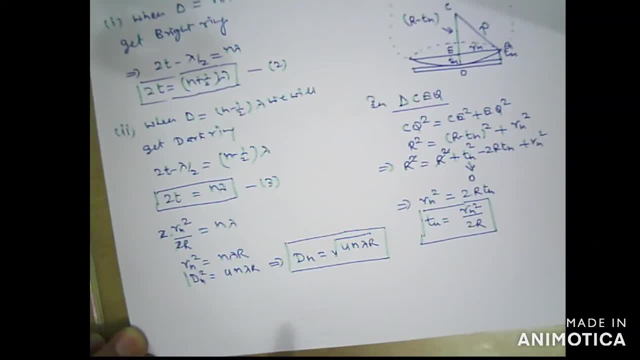 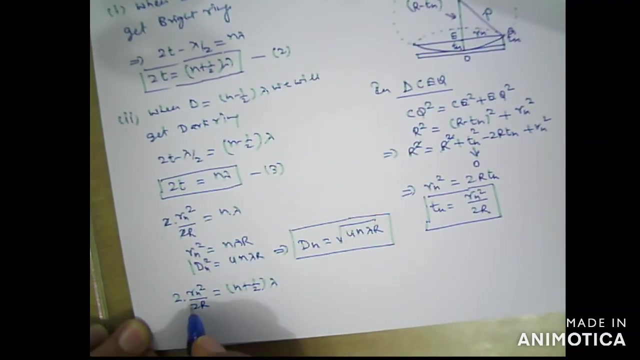 So if you put the value in equation number 2, you will get 2Rn square upon 2R equals to n plus half lambda 2 from 2 is cancelled, So Rn square equals to n plus half lambda R. 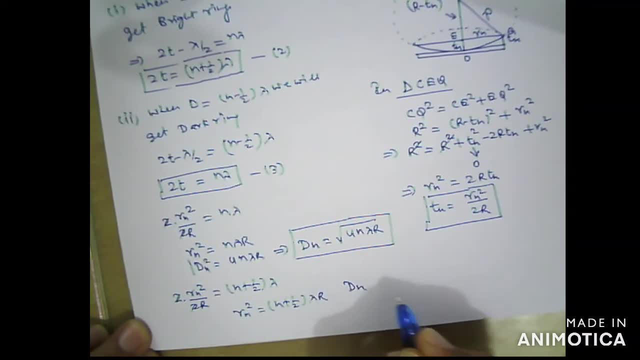 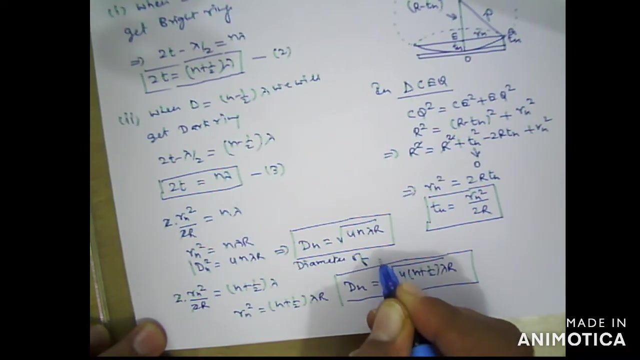 This is the value of the radius, And if we take out the value of the diameter from this, then how much will it be? dn equals to unroot 4n plus half lambda R. What can we write here? This is the diameter of nth order dark ring. 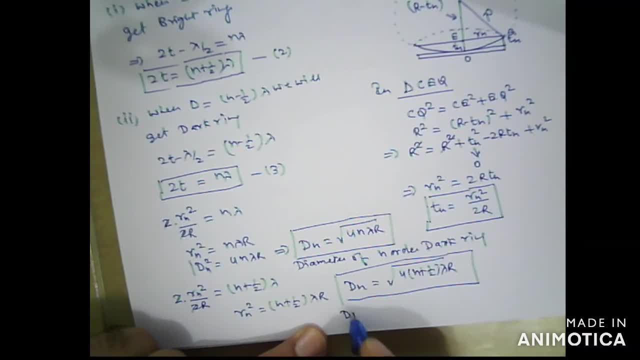 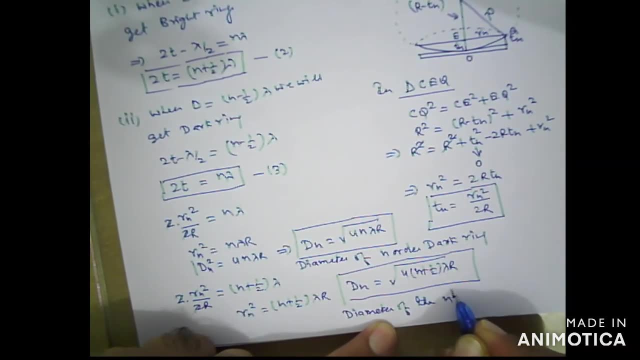 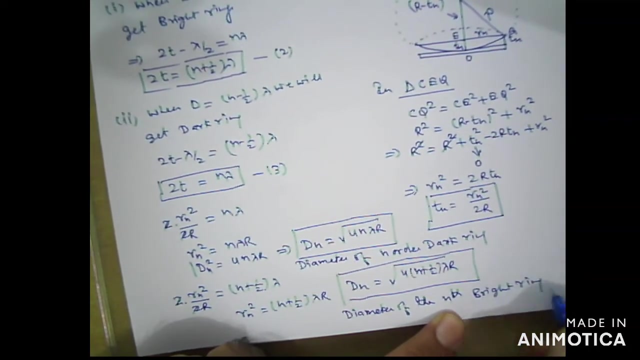 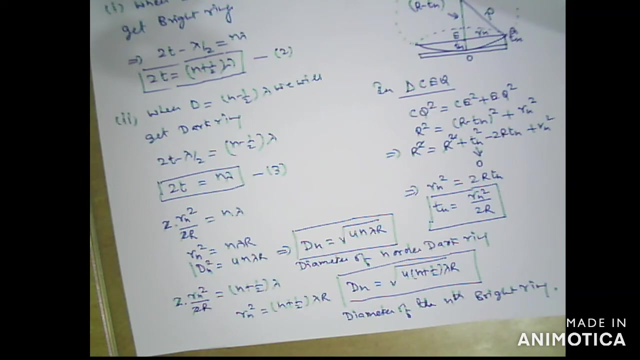 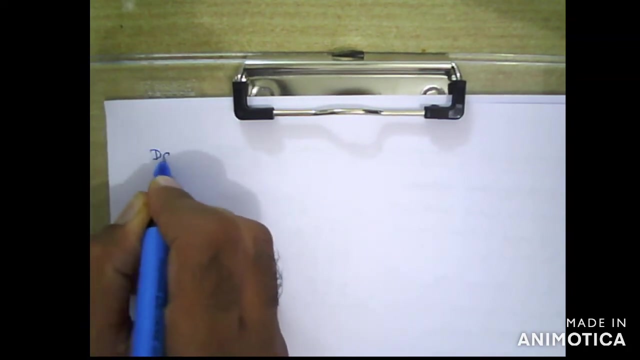 And this is the diameter of the nth order bright ring. So we have taken out the condition of dark and bright rings. So what is the formula of our dark ring? dark ring equals to dn, 4n, lambda R. If you write this formula, 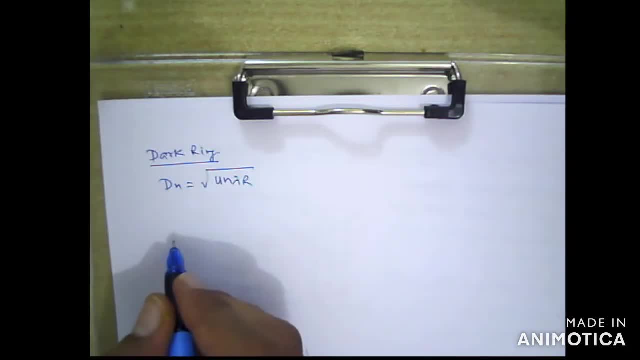 then you can get some conclusions. First one is that dn is proportional to the root n. That means if you increase the order of the ring then the diameter will also increase. But you will see that as the order of the ring increases, the diameter does not increase in that ratio. 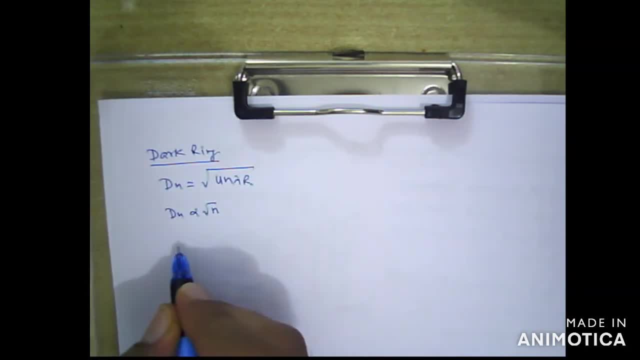 We can clear this with a small example: That root 3 minus root 2 is basically greater than root 19 minus root 18.. So the fringe width of the lower order fringes will be greater than the fringe width of the higher order fringes. 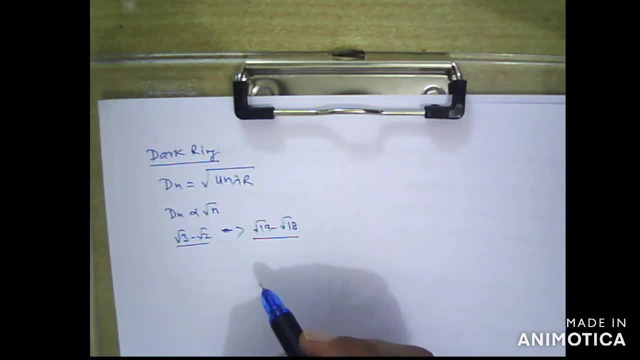 So the fringes of the starting order fringes. they have more space in them And as we move forward the fringe width of the fringes keeps decreasing. So now the next small topic in this is how the central spot is going to be formed. 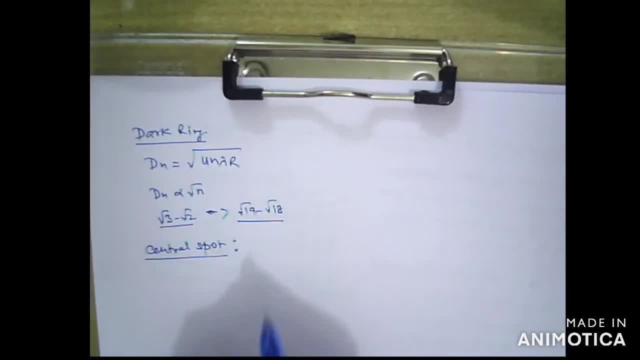 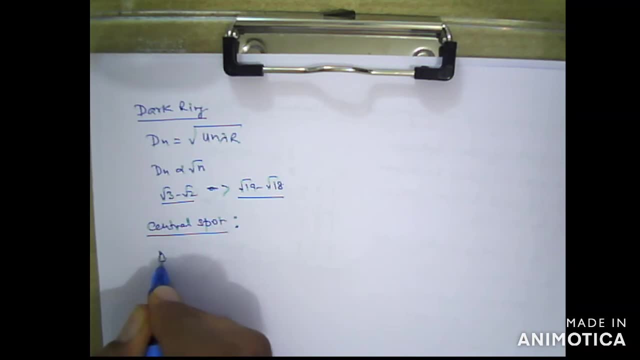 What about the central spot? So how the central spot is going to be formed. For that we will talk about. what was our path: difference 2, mu t cos R, minus lambda by 2.. So for central point, central point, t will be 0. 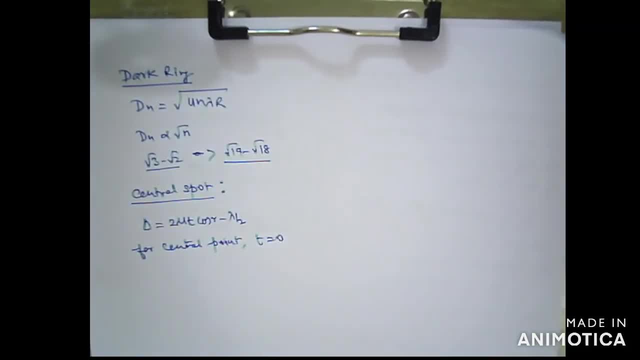 So for the central point, what will be the value of t 0.. If we write the value of t as 0, then what will be the path difference lambda by 2.. And if the path difference is lambda by 2,? 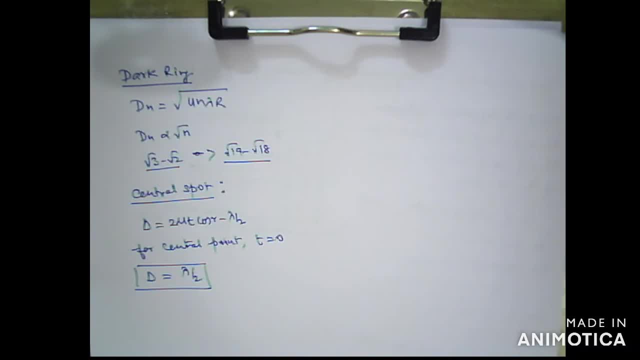 then what is the interference? Destructive interference. This means that the central point will always be dark. Now I will make a diagram in front of you. Suppose this was our glass plate, This was our plano-convex lens, which you had placed on it. 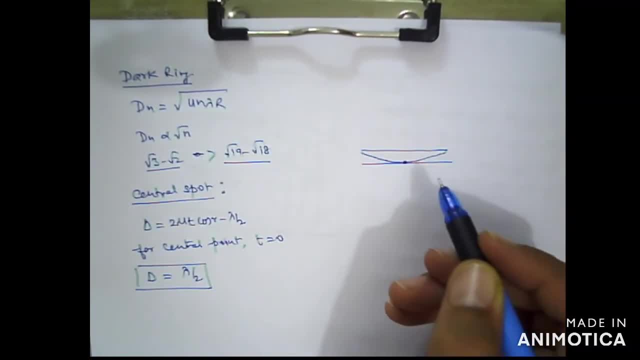 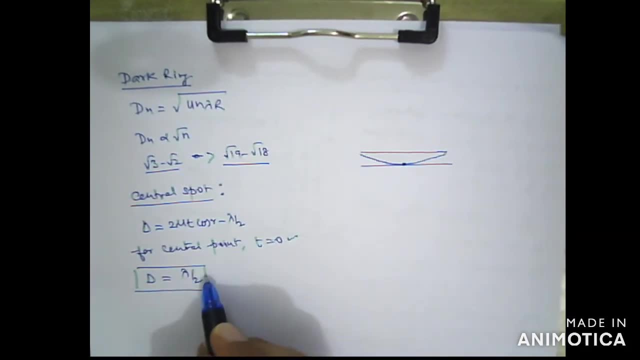 You can see that this contact point, which you have called the central point, is 0. Here the thickness of this film is 0. So if the thickness is 0, then what will be the path difference lambda by 2.. 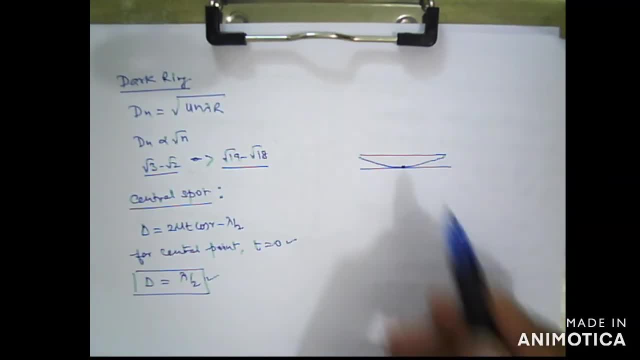 And if lambda by 2 is the path difference, then it will be a destructive difference. And how will the central point be formed? It will be dark. So when you look at it from the top of the microscope, what kind of reference pattern will you see? 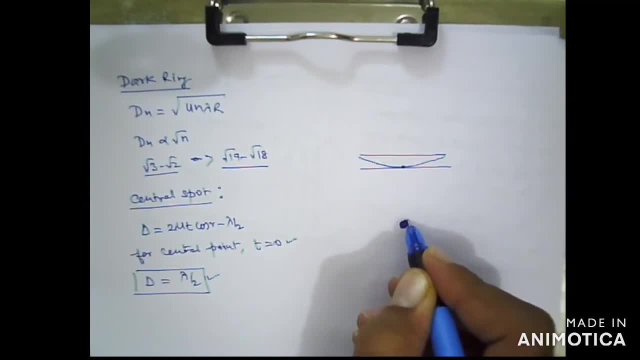 You will see a dark spot in the center And there will be circular rings around it. There will be concentric rings Like that. So if this is bright, then it will be dark, Then bright, then dark, Then bright, then dark. 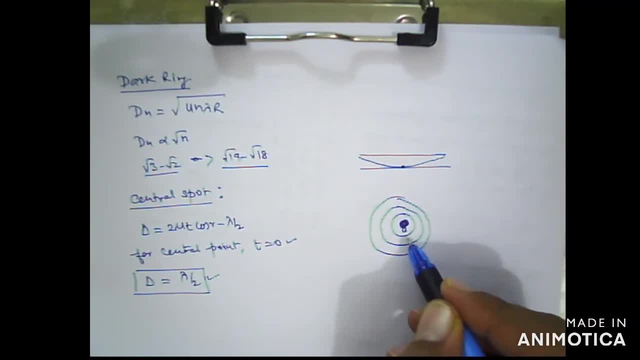 So the diameter formula of the dark and bright rings we have already calculated. So as the order of the rings increases, the rings will be closer to each other. The faster the rings come, the faster these rings will come. And when the high order is made, 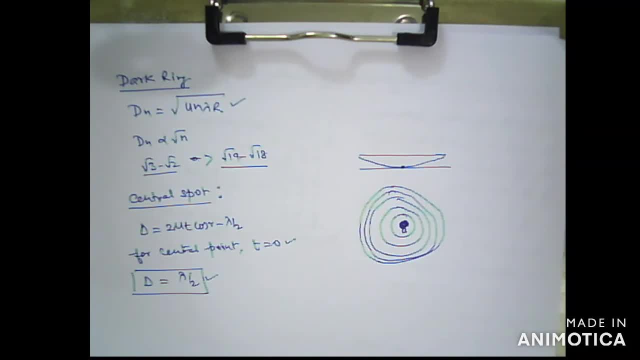 they will overlap to each other. The rings will overlap to each other. So this was the procedure for derivation of the diameter of the dark and bright ring. Now I will tell you how the questions come in the exam. So the questions that come in the exam are as follows: 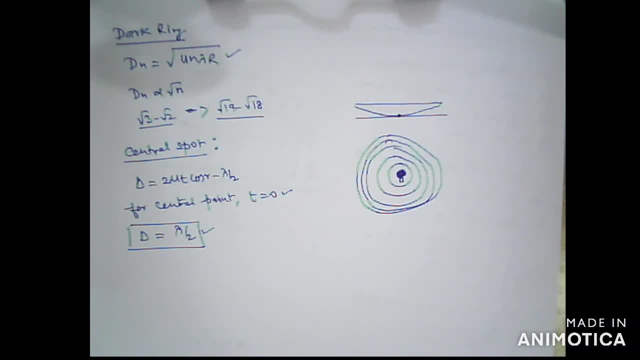 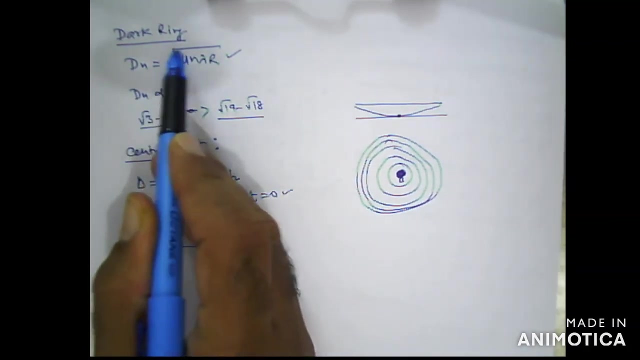 What is the Newton's ring And how you will prove that the diameter is directly proportional to the square root of the natural number. So here, like you, have taken the diameter formula of dn. So what is the answer? Unroot 4 is lambda r. 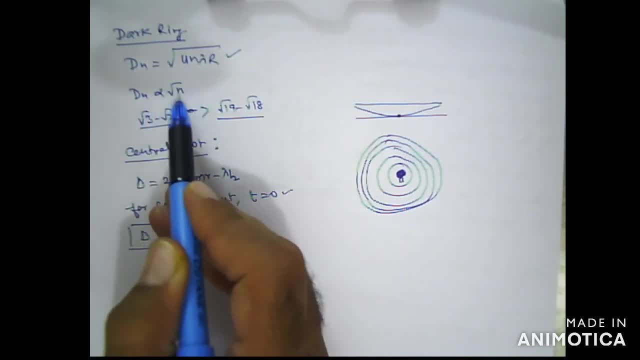 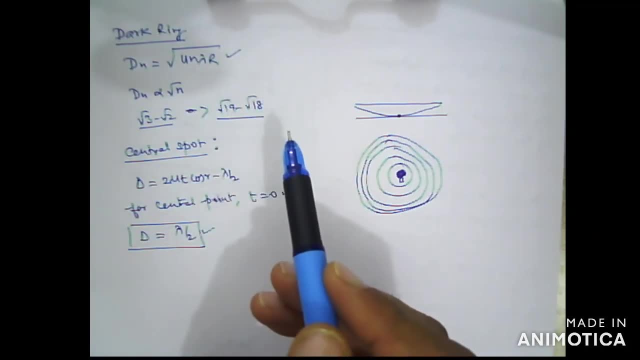 So from here you can see that dn is directly proportional to the root n. Okay, The second condition is that while we are keeping the radius of curvature, r is large. Why do we keep r large If you do not keep the value of r large? 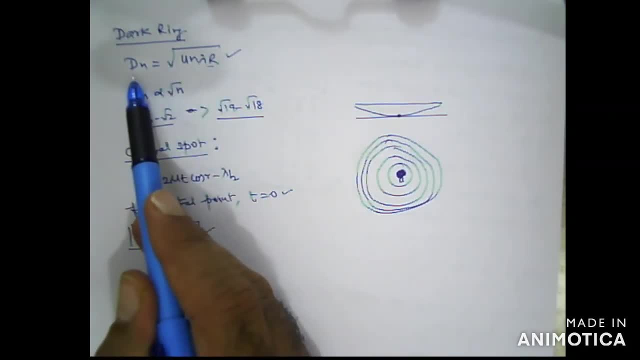 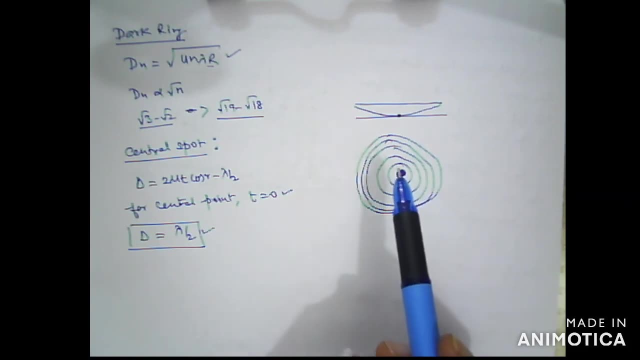 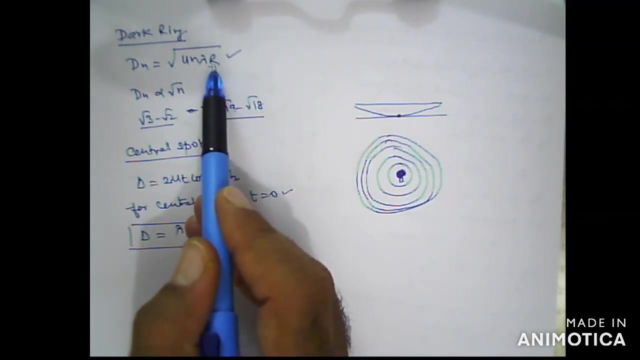 you will get the diameter of very few millimeters. How you will observe that Newton's ring fringes. If you want to observe spaced rings, then you have to keep the value of r high. If the value of r is not high, 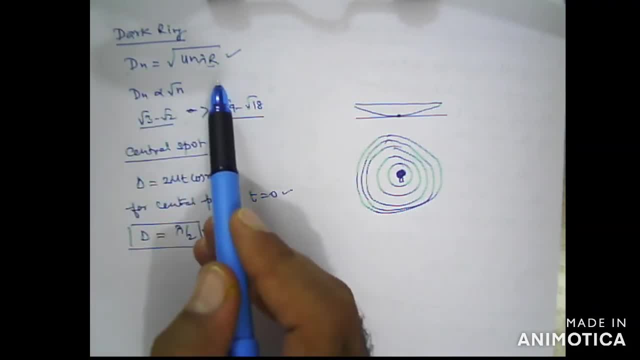 then the value of dn will be very low. That's why we choose the Plano convex lens of the large radius of curvature. So this is our derivation for reflected light. Similarly you can also make Newton's ring pattern for transmitted light. So in today's lecture,